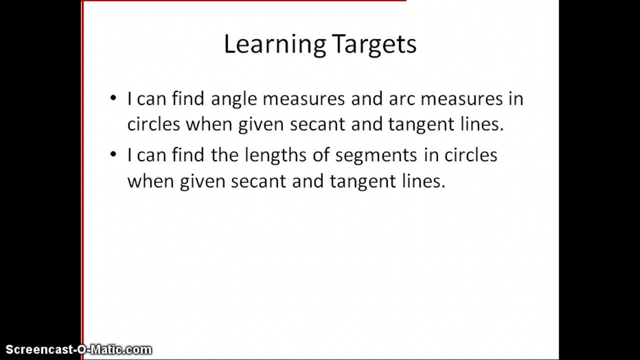 Hi. The second learning target for today is finding the length of segments in circles when you either have again a secant or you have a tangent line Again, secant lines go through the circle and tangent lines just touch the circle. Just kind of draw yourself. 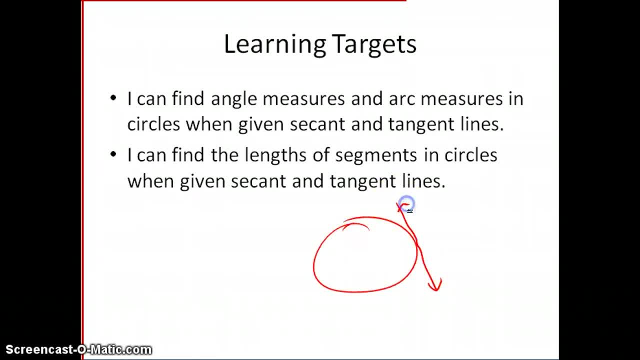 a picture again. Tangent lines touch the circle, secant lines go through the circle. So we're going to work on finding the length of segments for some of these today. Hi, So we have two examples here. This first example: again. notice that the lines are: 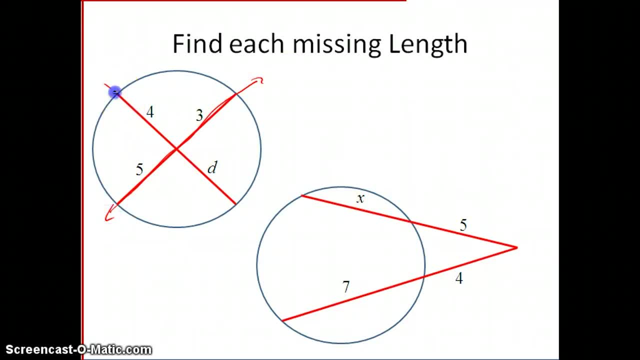 going through it. These are actually cords. The rule applies the same way as if you have cords or if you have secants. If the lines were extended, that becomes a secant. If they're shorter, it's becoming a cord. Again same thing here. If you extend these, that's fine. 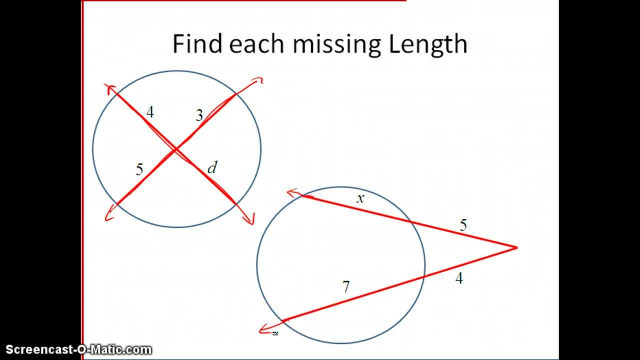 But it still has the same properties. Just like with angles inside and outside, you're going to have to find the length of segments that are going to reflect the length of the circle that you have. So you're going to need to find the length of the circle that's going to reflect the length of the circle. 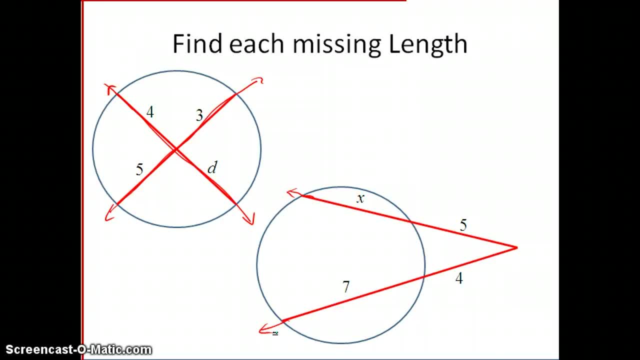 that you have right now. Let's think about that too. So if we have this first example, this circle here, this triangle and all the other triangles that are sitting here, both of these will have their own principles and they're very similar but again, slightly different In first semester. 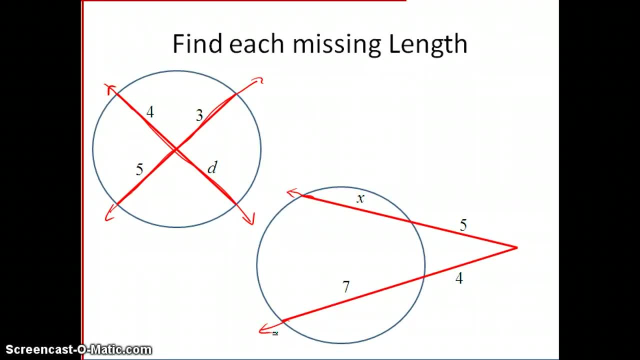 you talked a lot about similar triangles and you talked about proportions. We are going to be using that same concept today in the lessonSo when you look at this first example, you're going to use some proportions, the first example meaning this circle, Whenever. 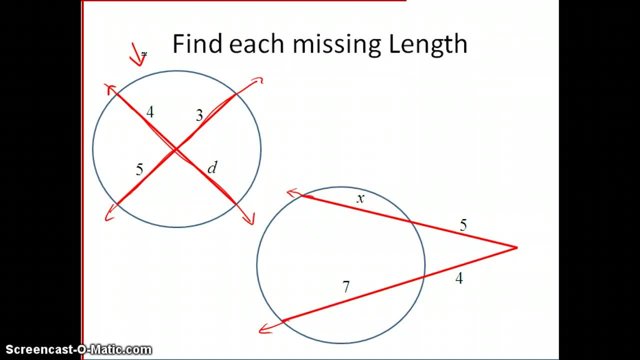 you have secants or cords that split up a circle and again it's not necessarily going through the center. you're going to have to find the length of the circle that split the segment. pieces are going to be proportional or kind of equal to each other. 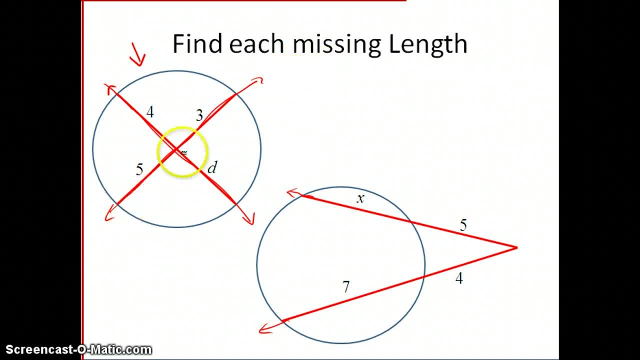 So what I mean by that is, we can set it up by saying: if I start with 5, I can do 5 times the other part of its segment. so 5 times 3 equals. well, then do the other segment, or chord, or secant, whatever it happens to be 4D. 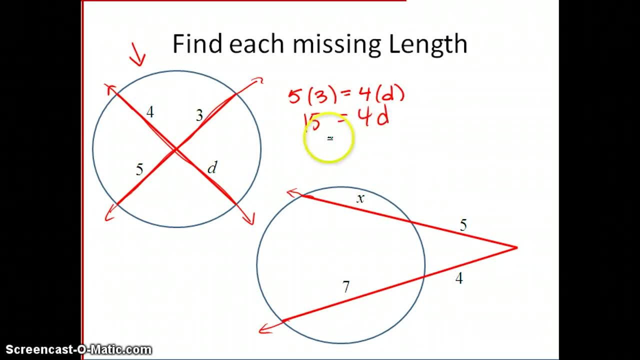 So you end up then just solving algebraically: 15 equals 4D divided by 4, and I'm going to write it just as a fraction: 15 fourths. So when it's inside again, principles are different for inside and outside. 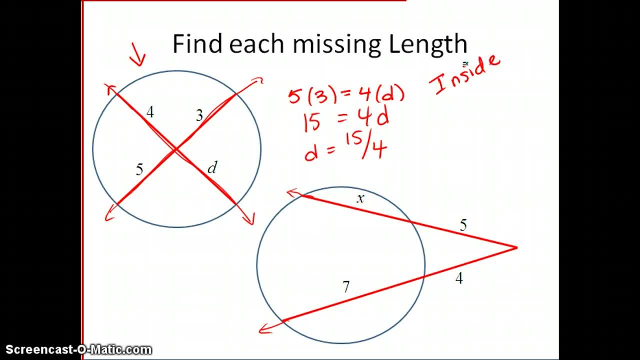 just like angles, When your chords, when your secants intersect inside and you're trying to find length. this is going to be the hard part: distinguishing between length and angle. read very carefully. If it's inside, you're just taking- and I call this A. 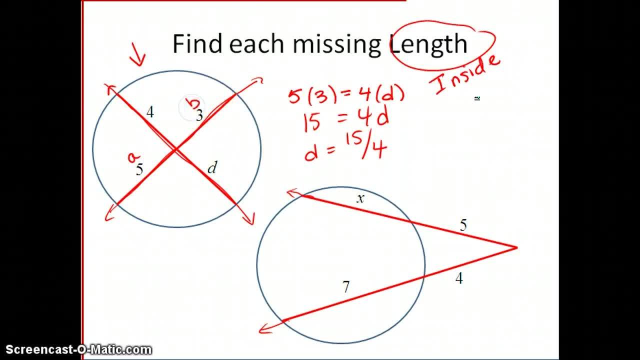 and I call this one, I think, B on the previous slide It's just A times B equals C times D, And that works every single time for finding length when secants or chords intersect inside a circle. The second example I have over there is where the secant lines 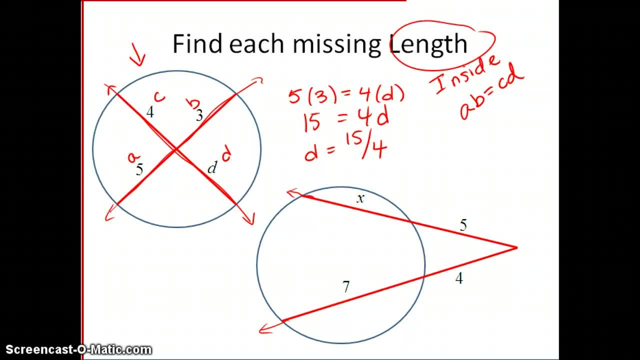 or the rays. again, it doesn't matter if it's a secant line or if it's a ray. if they intersect outside the circle they have a different property. And this one's a little bit, It's a little bit harder to explain, but again, 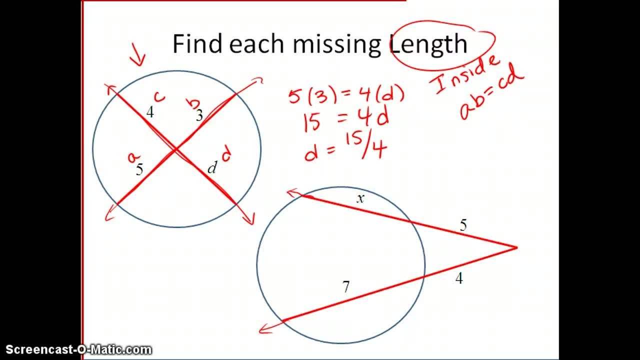 it goes back to similar triangles and proportions that we learned about earlier in the year, But the property for this one is: you always look at what's on the outside first. So 5 is on the outside of that top ray or top segment, And then you have to multiply it by the total. 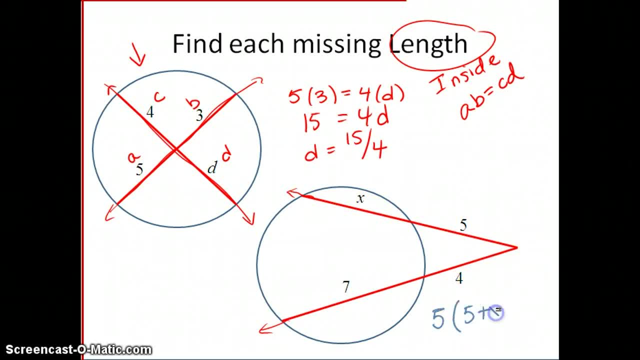 Well, how do I find a total That would be 5 plus X? Because I just have to add them together to find the total And, just like before, equal the same thing on the other segment, The outside is 4.. And then you have to multiply it times the total 4 plus 7.. 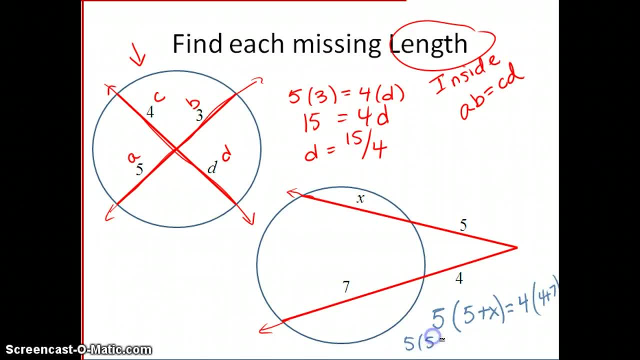 Now, hopefully you were able to do that- 4 plus 7, and write down 11.. So you have 4 times 11. And you can make that 44. And then really, what happens is you use your distributive property. 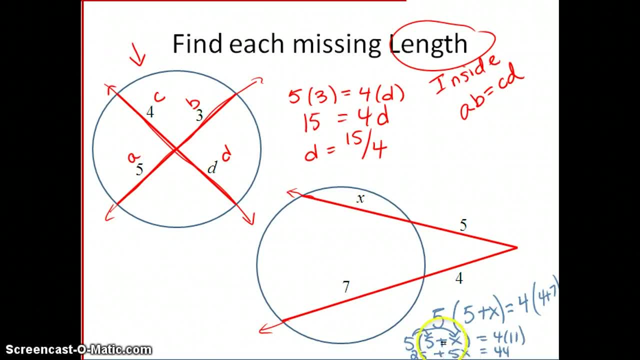 So you have 25 plus 5X, Subtract your 25.. I'm sorry, I'm running out of time, I'm running out of room. So I have 5X, equals subtract 25 from 44, I get 19..